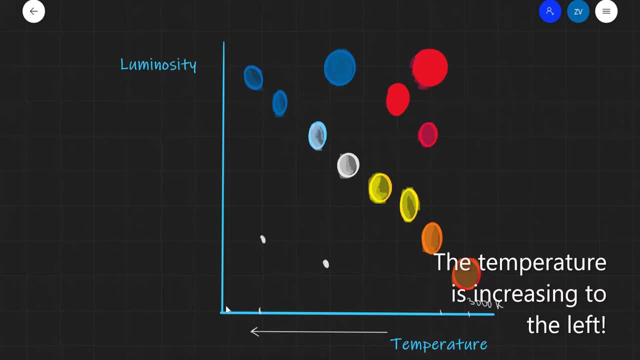 temperature on the surface of the star and over on this end, we have 30 000 plus Kelvin. So let's just say 30 000 plus Kelvin. over on the left end, On the y-axis, we have the luminosity of the star, which is a measure of the total power which has. 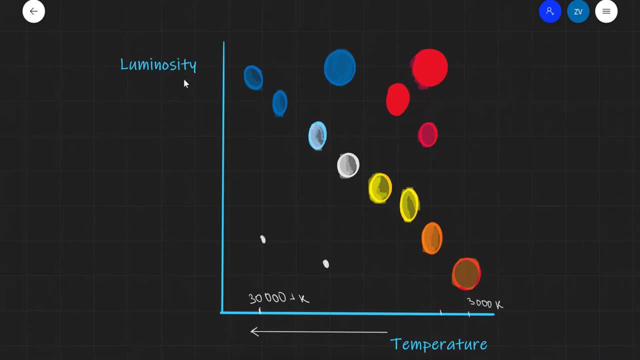 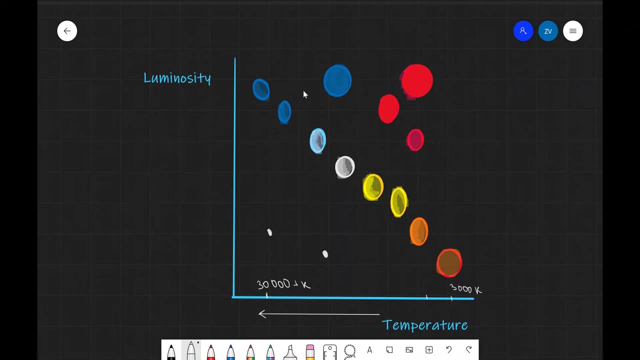 been radiated by the star. What are the main features on the diagram itself? First of all, we're going to notice that there's a clear diagonal line over here, So I'm even going to highlight this. but this section over here is known as the main sequence, So we can write this: 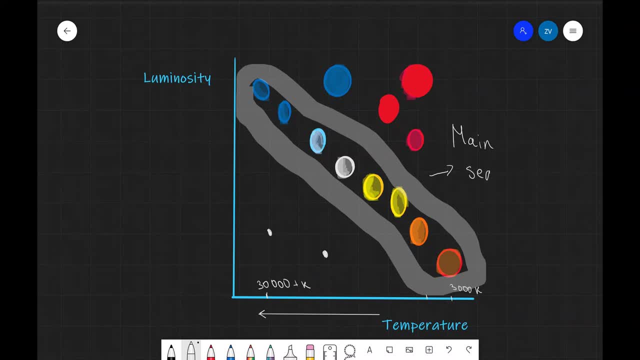 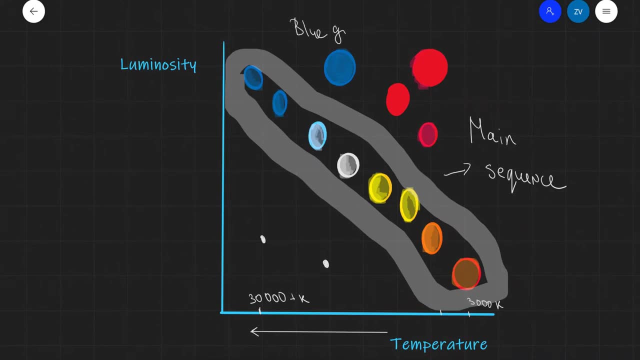 down that this over here is the main sequence. on the left We have blue giants, So we can write, and these are super blue giants in particular, and these are super red giants, like so, and just below them we can find the red giants. notice that the color of the star. 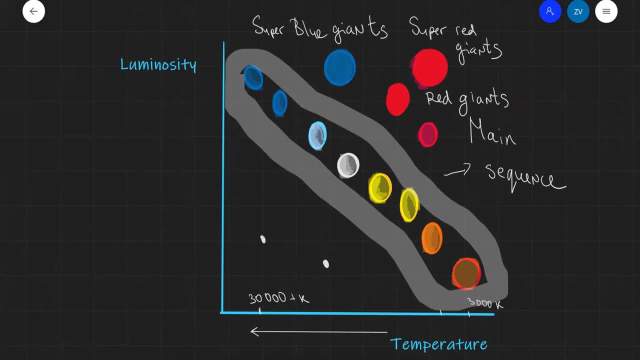 corresponds pretty accurately to its surface temperature. for instance, the stars which are on the right hand end tend to have a lower temperature and they have a red color. the reason for that is that is because red has the longest wavelength, and remember that the energy of the particles of light, called photons, is actually inversely proportional. 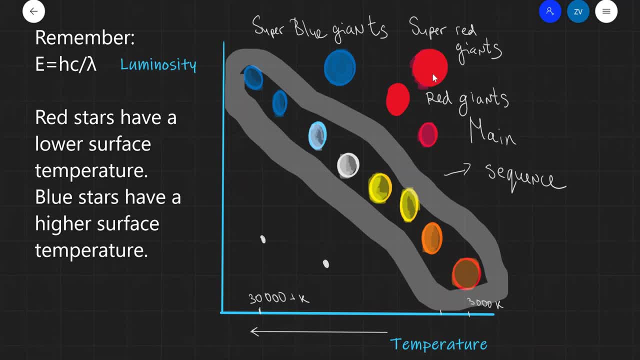 to the surface temperature of the star. so that means the energy of the stars is mostly proportional to the surface temperature of the star. so that means the energy of the stars is to the wavelength. so that means that the longer the wavelength, the lower the temperature. so red with a long wavelength is found on this portion of 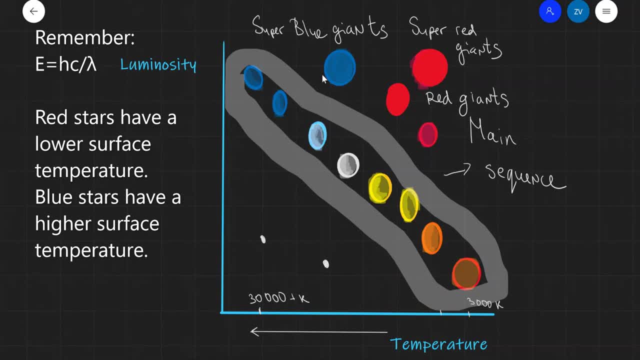 the graph. whereas blue- with a very short wavelength it has- the stars with blue color have a very high temperature. finally, notice that here on the in the left-hand corner of this diagram, we are going to find the white dwarfs and we can write this in. so this over here is the region for the white dwarfs, like so.